Hello, welcome to MooMooMath. In this video I would like to talk about edges, vertices and faces of a solid. The face is the flat surface of a solid. The edge is where the two faces meet. The vertices is a point where two or more edges meet. If your solid is a 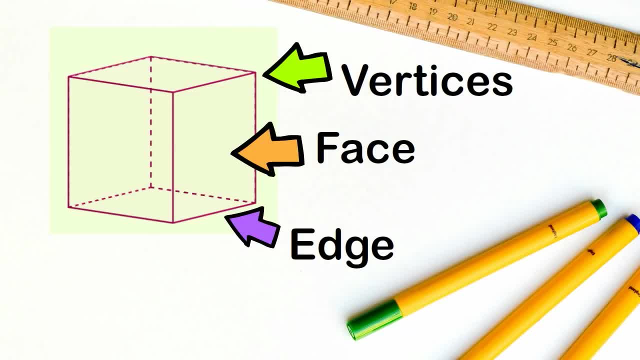 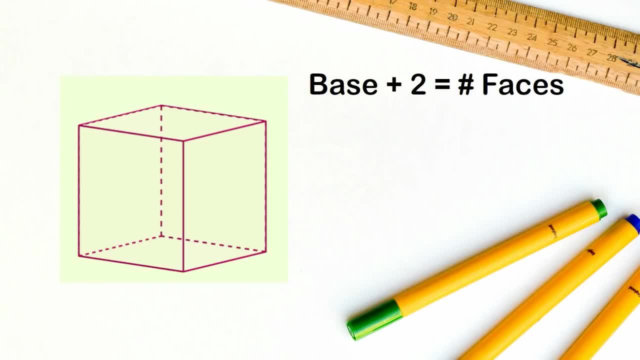 rectangular solid, then you can use a simple formula to find the edges, vertices and faces. The base plus two equals the number of faces. The base times two equals the number of vertices. The base times three equals the number of edges. This cube is a rectangular solid and 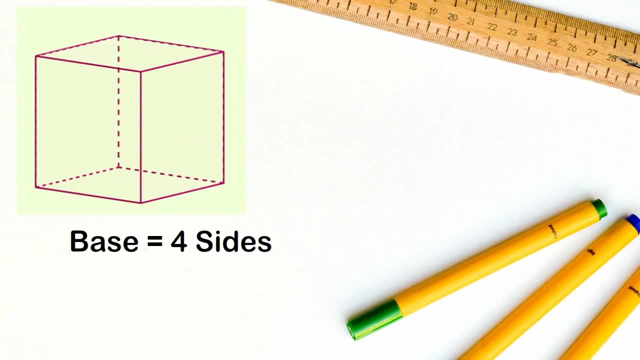 has a base of four sides. Four plus two equals six. the number of faces. Four times two equals eight, which is the number of vertices. Four times three equals twelve the number of edges. Unfortunately, you can't use this for all solids There is. 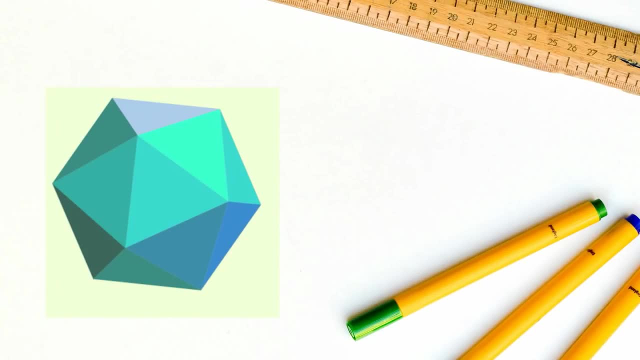 another formula you can use for all convex polyhedrons. It is called the Euler's formula, used in geometry. It states: the face plus vertices minus the edges equals the edges. Let's look at some examples of Euler's formula. This cube has six faces plus eight vertices. 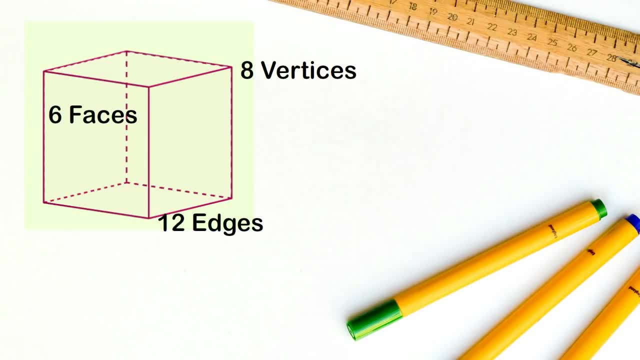 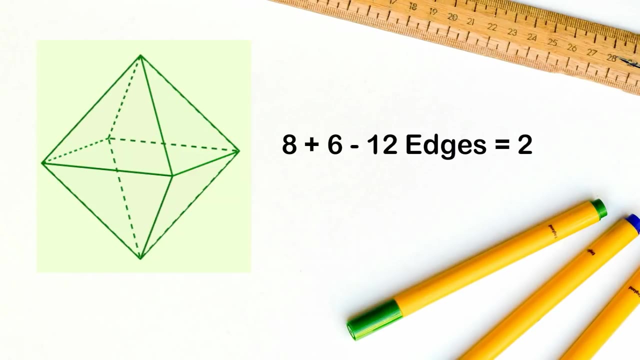 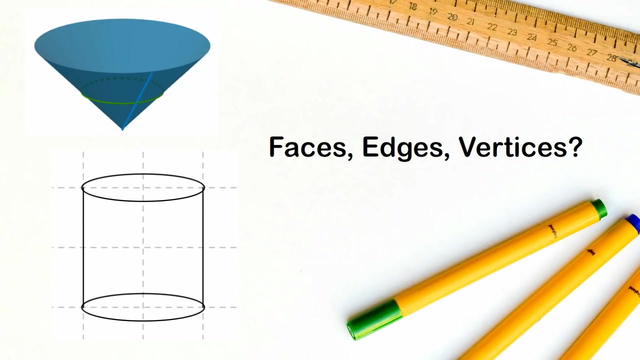 minus twelve edges, which equals fourteen, minus twelve, which equals two. This octahedron has eight faces, plus six vertices, minus twelve edges, which equals two. What about a cone or a cylinder? How many faces and edges and vertices do these have? If your definition of the face will allow for a curve, then the cone will have two faces. 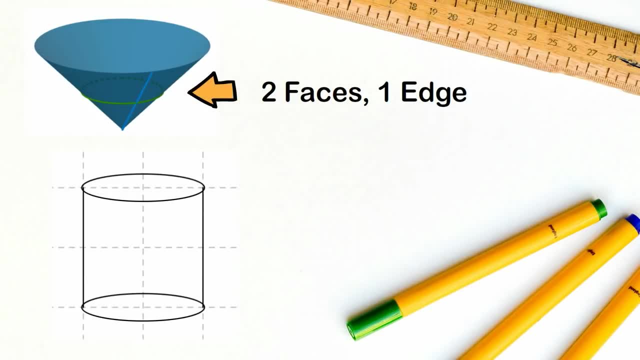 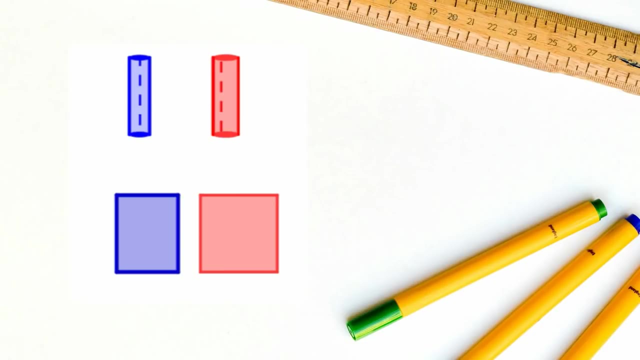 and one edge. The solid cylinder will have two edges- if you allow the edge to be curved- and three faces: Two circular ones and a rectangle. If you take the top and bottom off of a tin can then cut the cylinder part on this seam and flatten it out, you will get 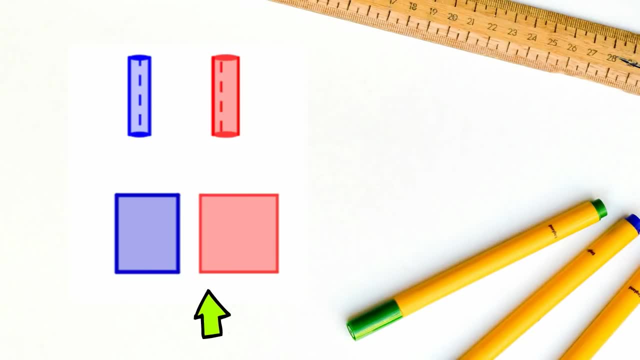 a rectangle and no vertices or corners. Thanks for watching. I hope this helps with edges, vertices and faces. MooMooMath uploads a new Math video every day. Please subscribe and share.